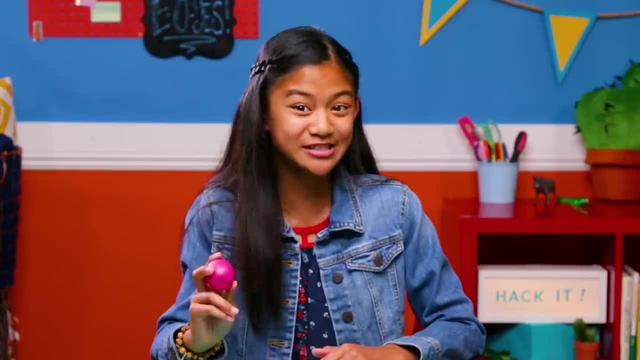 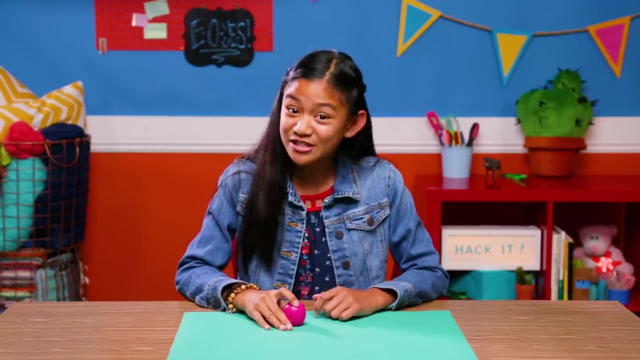 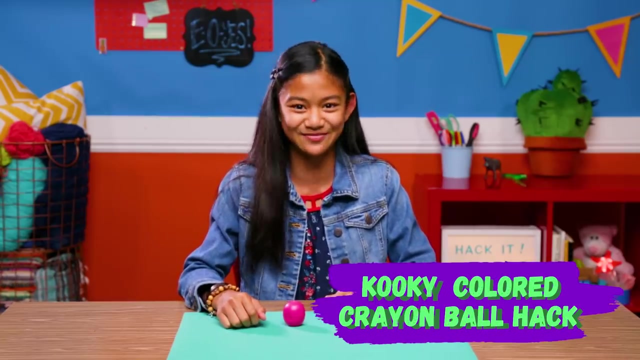 I'm going to hack some supplies from my leftover EOS containers. That's why today's episode is My Handy Dandy EOS School Supply Hacks. My first hack takes one of these old chapstick containers and turns it into a colorful writing utensil. Let's make my cookie colored crayon ball hack. 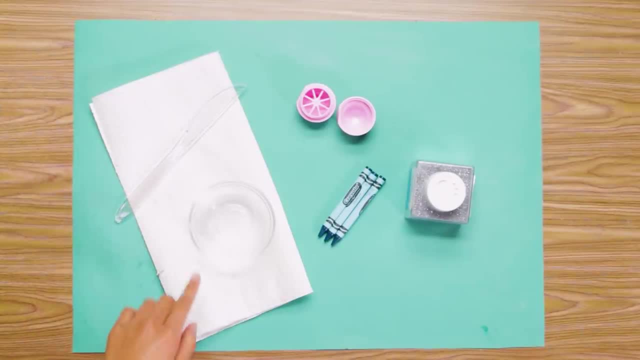 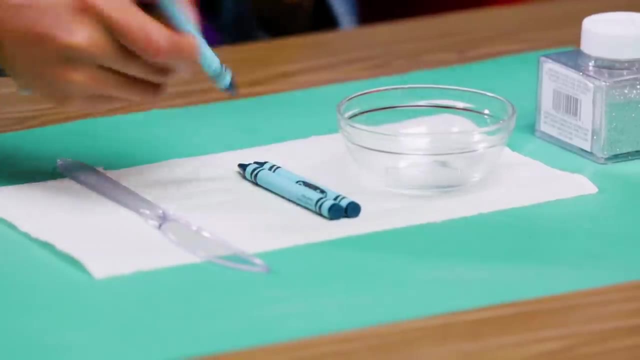 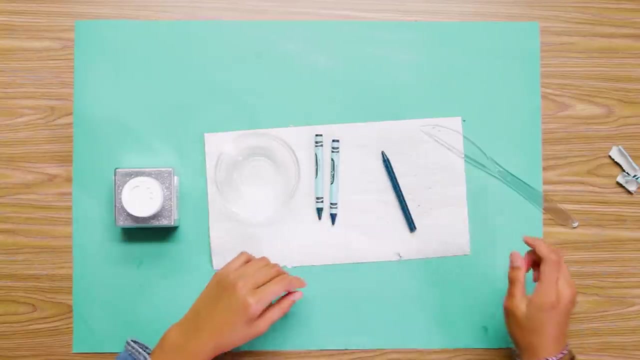 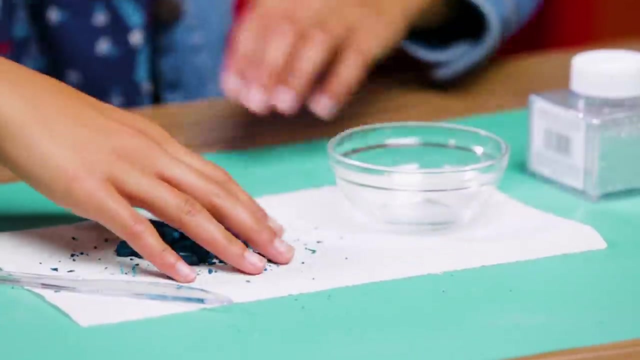 For this you'll need a plastic knife, a paper towel, a glass bowl, three crayons, glitter and an empty EOS container. First, remove the paper from your crayons Carefully. cut your crayons into little pieces, Put them into your small bowl and add some glitter. 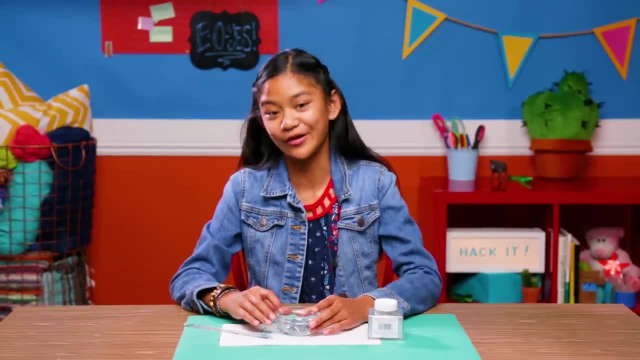 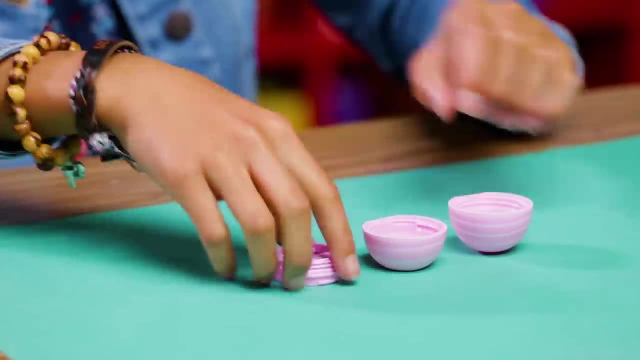 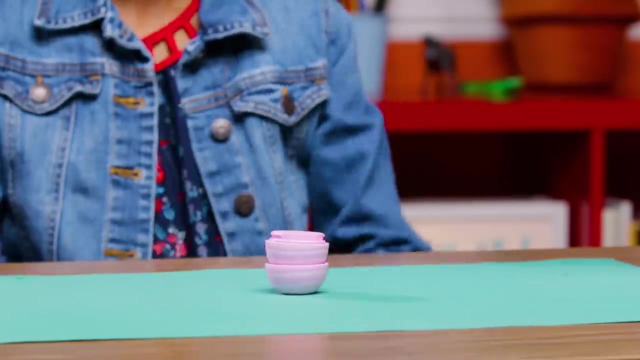 Melt your crayon and glitter in the microwave for about three minutes. Now remove the middle piece of your empty EOS container. Screw this into the top piece. Set the container aside. Put this in the bottom piece to help it stand up straight. 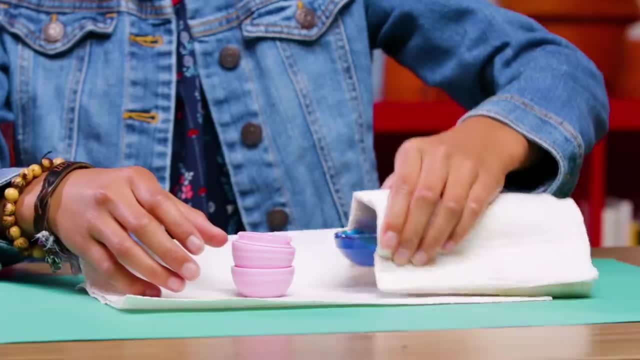 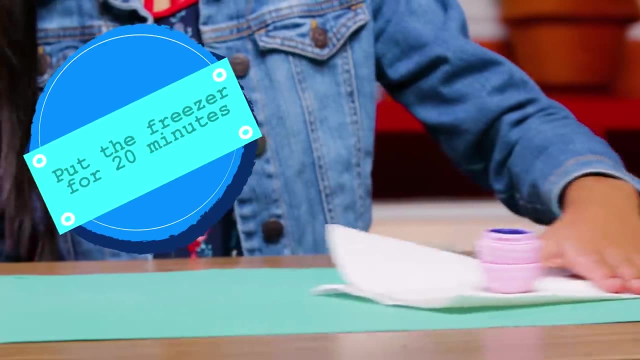 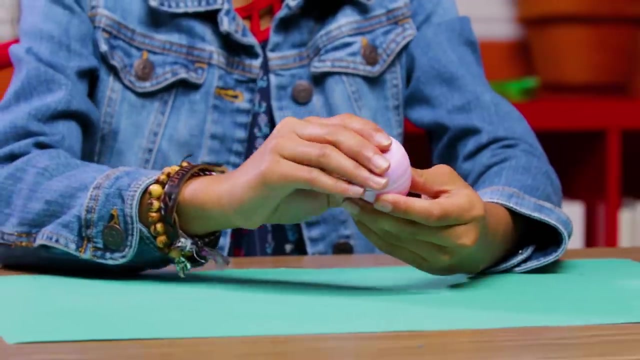 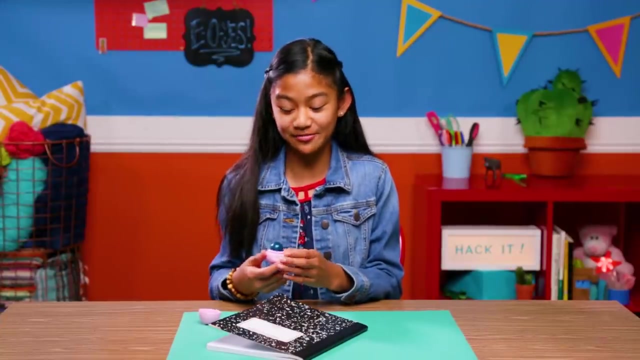 Careful, this is really hot. Use a paper towel to carefully pour your melted crayons into the EOS container. Now put this in the freezer for 20 minutes, Pop the bottom back in, Then unscrew the top. Ta-da, Now I can doodle in style. I mean, take notes. Now I can take notes in style. 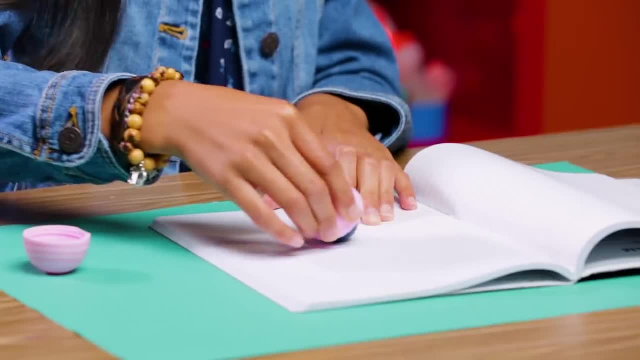 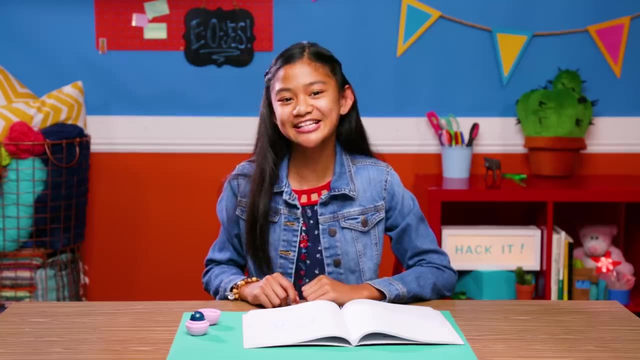 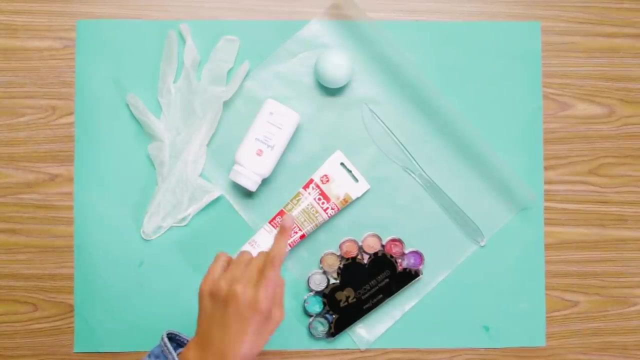 I've got more than a cool compact crayon up my sleeve. It's time for my next hack, my easy eraser hack. For this you'll need gloves, baby powder, silicone, old eye shadow, a plastic knife, an empty EOS container and some wax paper. 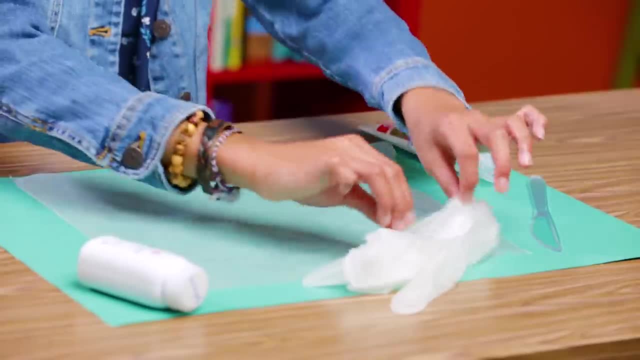 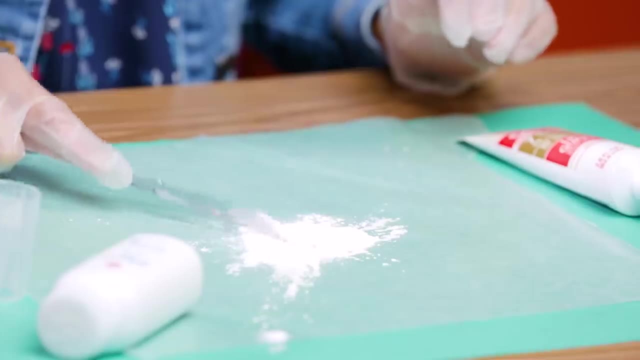 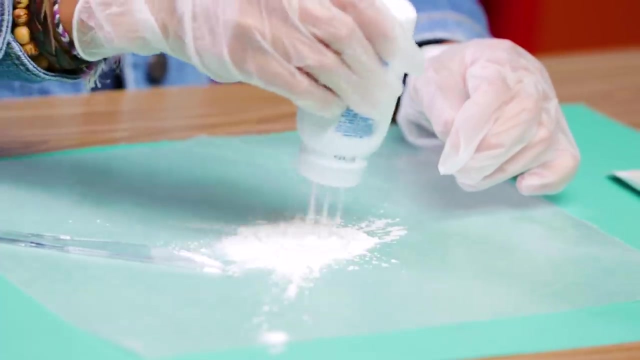 Open your empty EOS container like you did before. Put on your gloves, Lay out some wax paper, Then pour some baby powder on top and smooth it out into a wide circle. Now add your silicone on top in a spiral. Then put some more baby powder on top. 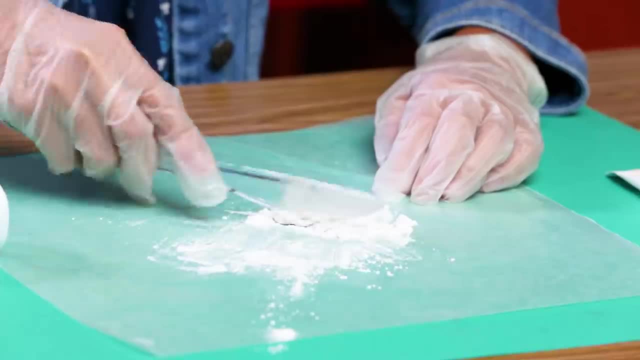 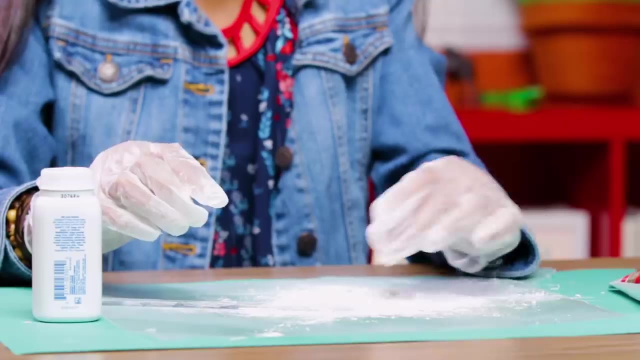 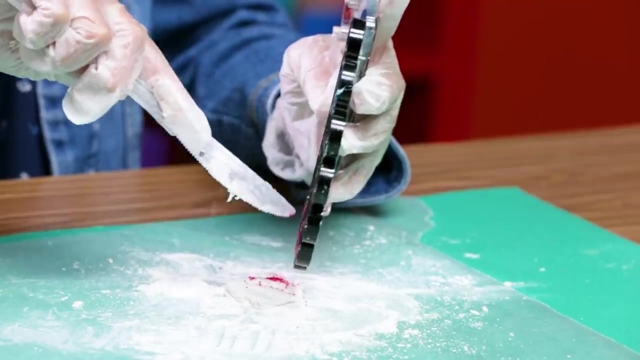 Use your knife to help completely cover the silicone with the baby powder When it starts getting clumpy. use your hands to roll the dough into a ball. Flatten out the ball. Pour some eye shadow on top, Mix it together completely. Form it back into a ball. 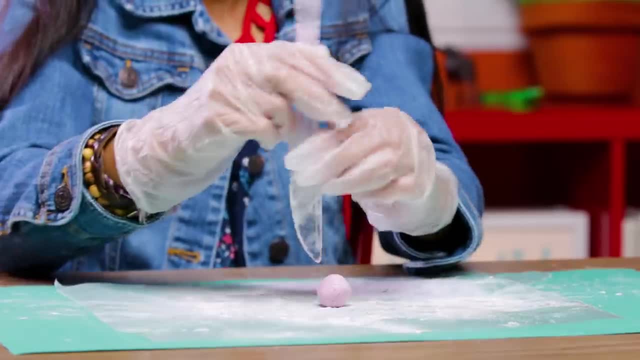 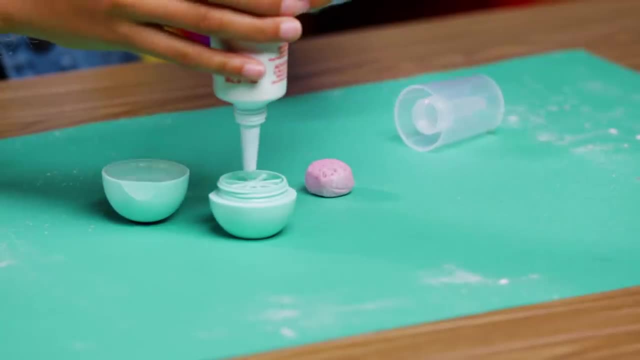 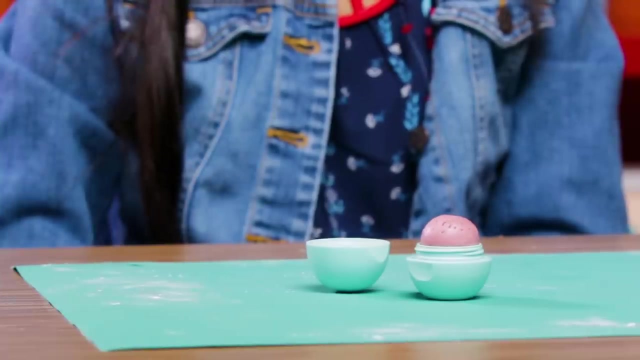 Use your knife to poke holes in the ball like this. Let it sit for 10 minutes. Dab some silicone on the grid of your EOS. Place your eraser gum on top. Let it harden overnight. This eraser is so cute. 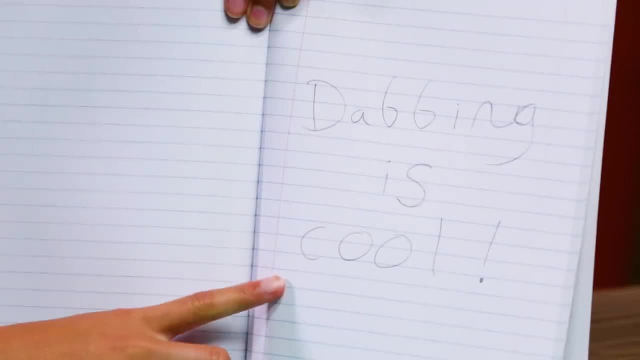 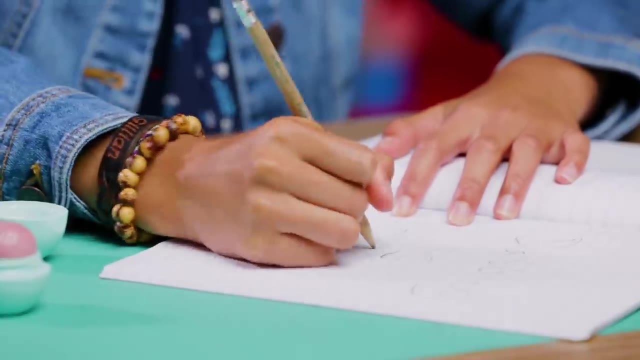 You won't feel so bad when you have to erase those big marks. It will help you get rid of the mistakes. Now I have one final EOS hack for you guys. It's time to turn your boring USB port into a fashion statement. Let's make my USB diva drive. 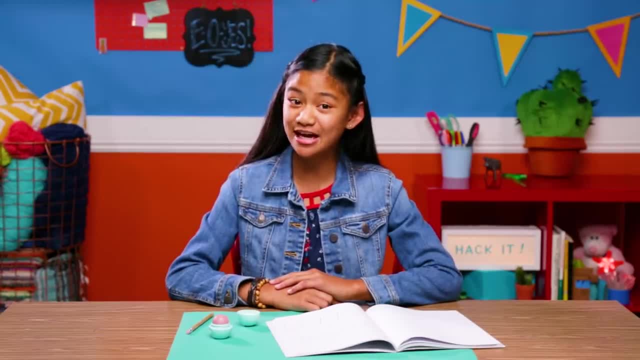 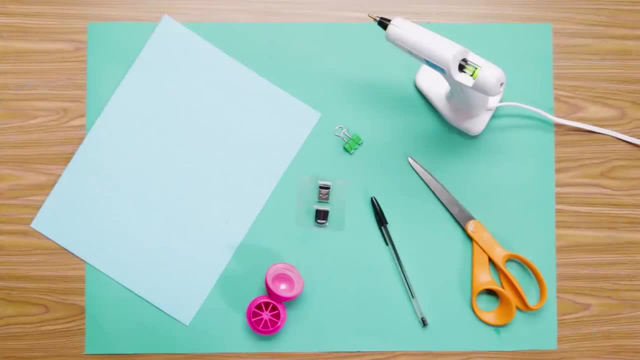 For this you'll need felt, an empty EOS container, a mini USB, a binder clip, a pen, scissors and a hockey stick. I'm going to use a small size USB stick. I'm going to use a small size USB stick to hold the EOS in place. 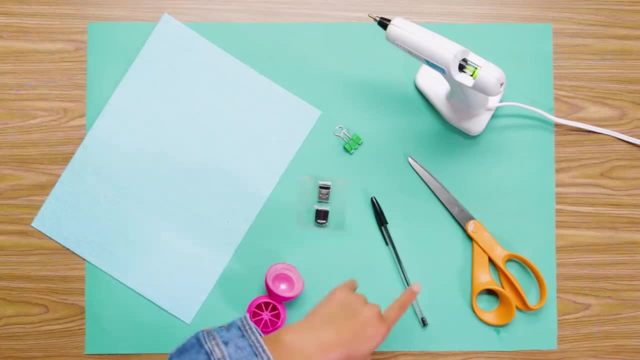 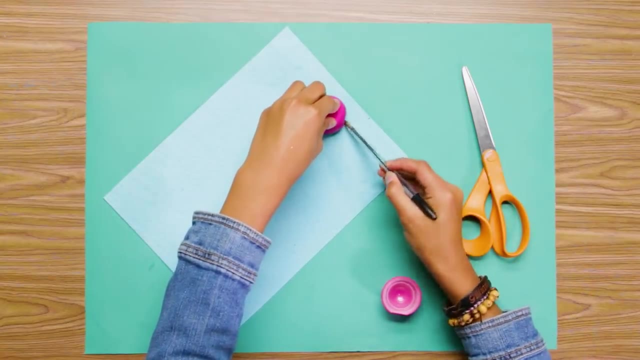 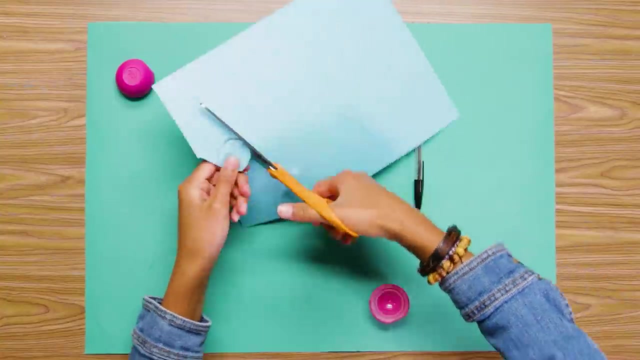 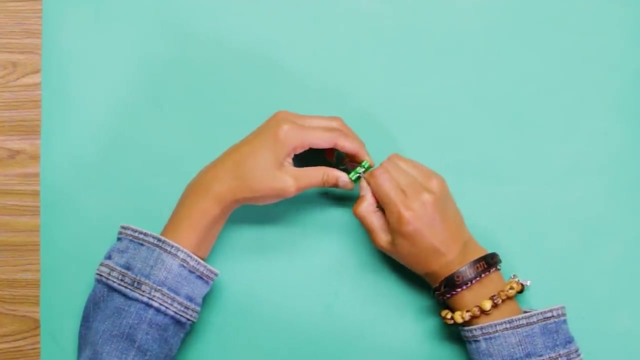 I'm going to use a small size EOS stick to hold the EOS in place, A pen, scissors and a hot glue gun. Trace the bottom part of your felt. Cut that out inside the lines, Put it aside. Remove one of the metal handles by squeezing it like this. 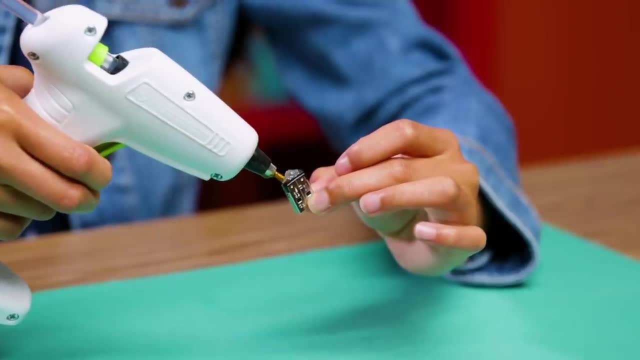 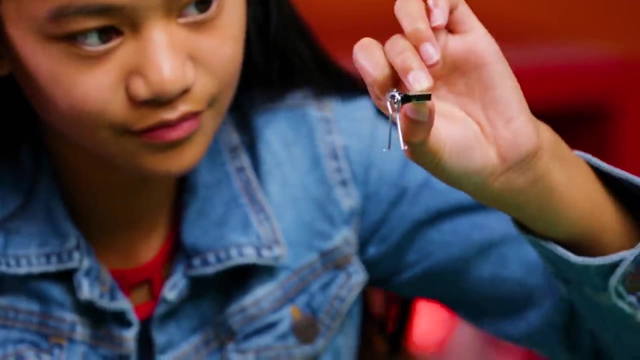 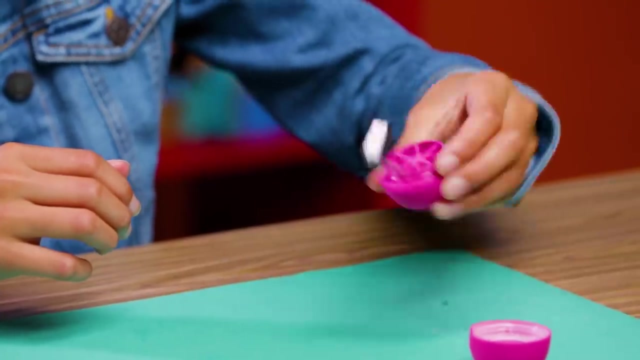 Now glue the bottom of the USB to the round part of the handle, making a right angle. Grab the bottom piece of your EOS and your binder clip. Pinch the ends of your binder clip and put it through two of the grates like this. 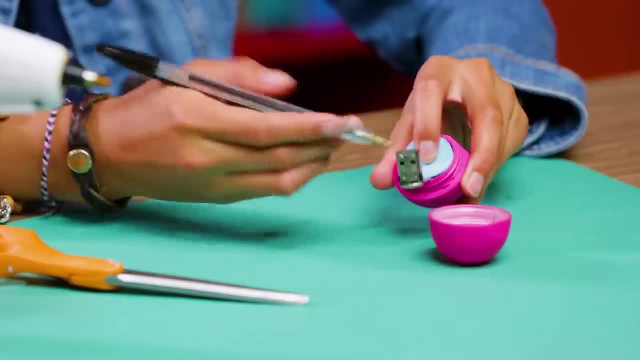 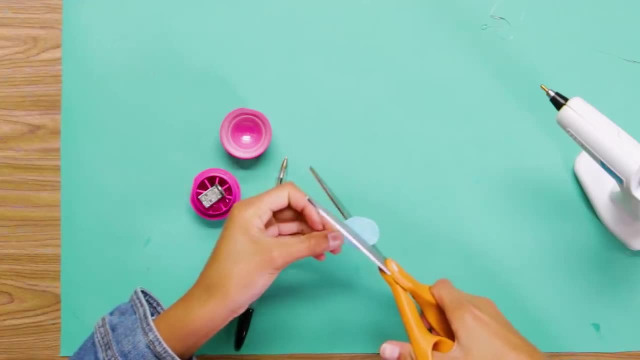 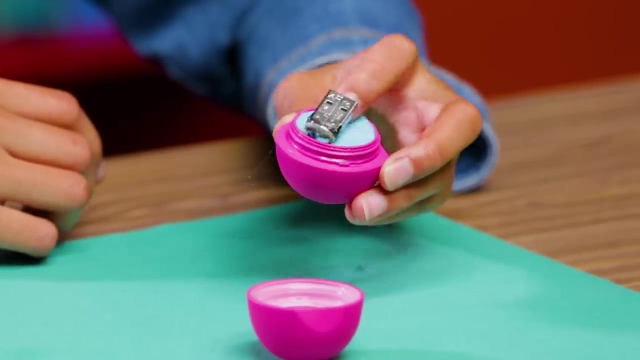 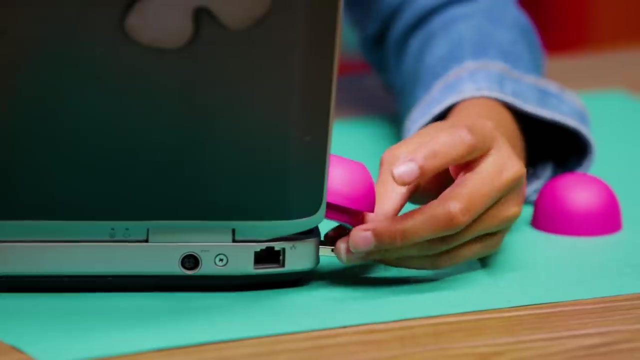 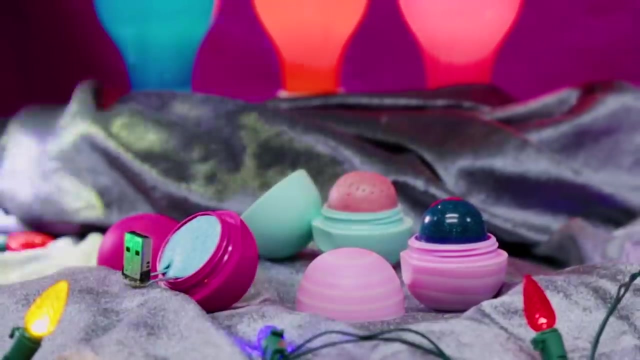 Grab your piece of felt, Put it on the grate Mark and cut two slits for the clip. Now glue this on avoiding the metal: A USB port hidden in a stylish compartment to protect all my secret files. Say bye-bye to your old school supplies with these awesome EOS hacks. 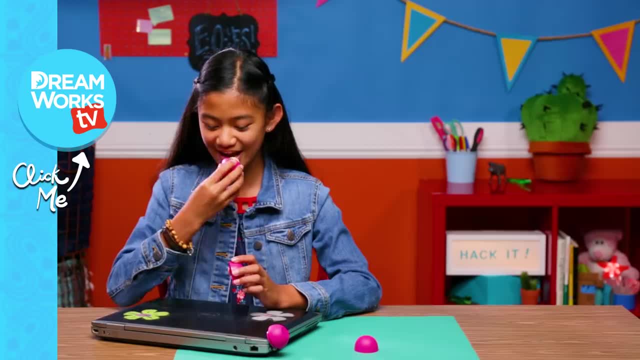 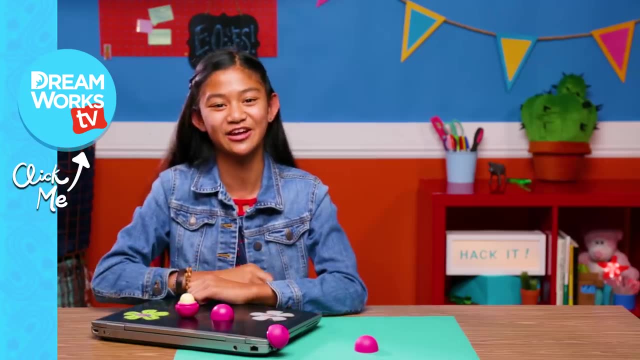 Thanks for watching. Remember to subscribe to DreamWorks TV and click here for more life hacks for kids. Let me know in the comments down below which EOS hack is your fave. See you next time. Bye for now.